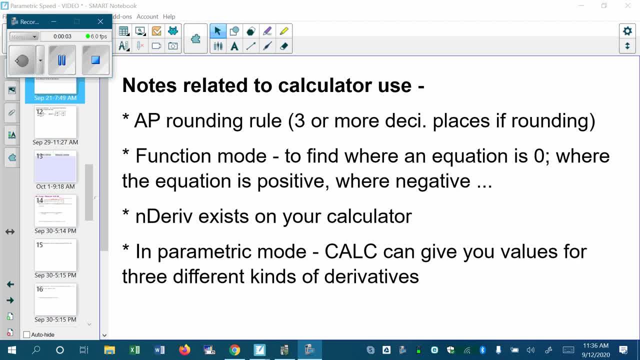 Hi. so this video is about parametric speed, but it also is an overall review and a couple of important comments. So I had in my notes from last school year that my students last year had some issues with calculator use at this juncture, And so I decided to include in this video a few comments about calculator use. 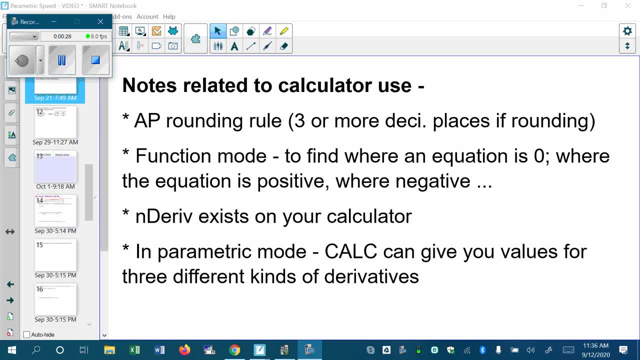 So my 1st bullet point on the screen right now is just to make sure that you're all cognizant of the fact that there is an AP calculus rounding standard, and it's not even as complicated as in science when you have significant digits or something like that. 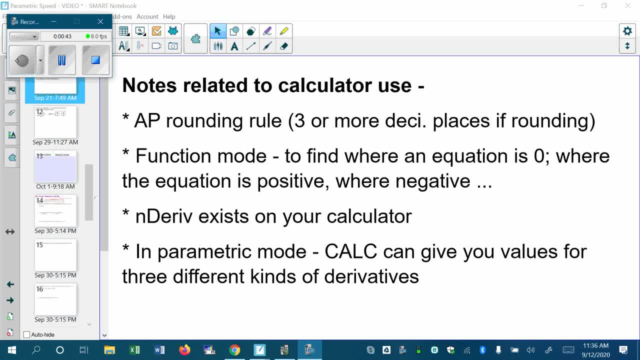 It's. it's just way more basic than that. And so if you go to the decimal point, and then there's the tens, hundreds and thousands place, it's to round to the nearest thousandth. If you are Are rounding, so if you're not, well, you don't need to worry about this at all. So don't start saying: okay, my answer is 5. so now I have to write 5.000.. that is not what we're talking about. 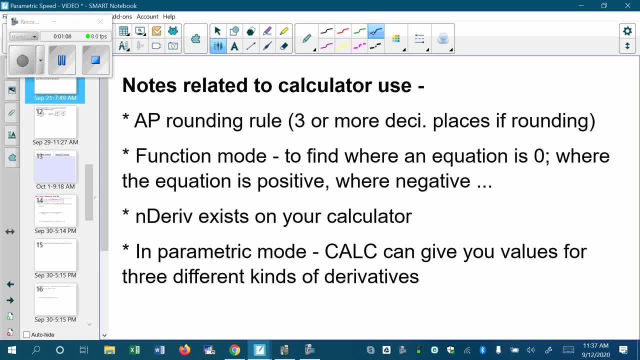 We're saying, if you indeed are rounding an answer, that you need to include the decimal point and then 3 digits after that. Now, the 3 digits can either take into account what comes in the 4th decimal place, and you can round up or down based on. 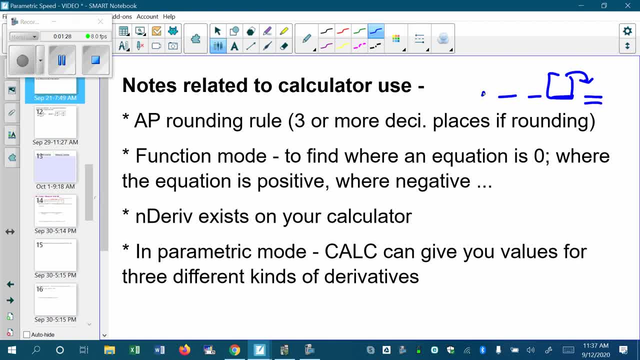 That's the decimal place where I actually would prefer, and what I would coach you to do, is just to truncate. Just needs to chop it off. So right, decimal point, digit, digit, digit. stop. Both the rounded version and the truncated version will be accepted. A version where you give fewer budgets than that will lose you the answer point. 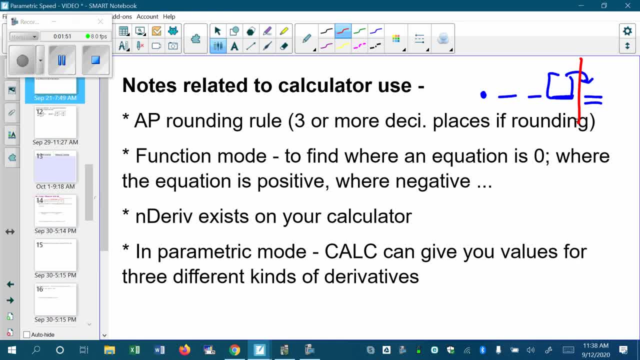 The 2nd point up here is to remind you- and this is something that I commented on in the previous video that I recorded- is that just because you're doing a parametric type question, something in the parametric context, doesn't mean your calculator has to be in parametric mode. 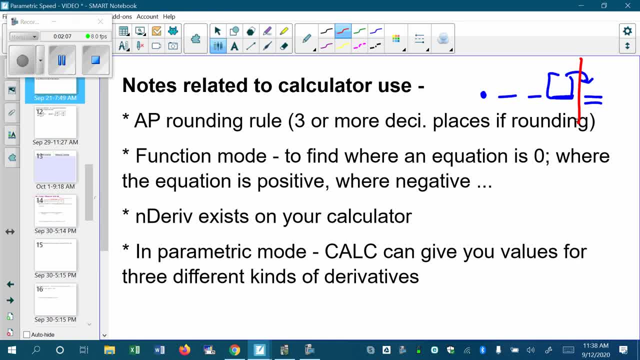 You might be in function mode. So function mode is used to find where an equation is 0, where an equation is greater than 0, where an equation is less than 0. So function mode is definitely something that can be utilized, regardless of what context the problem comes from. 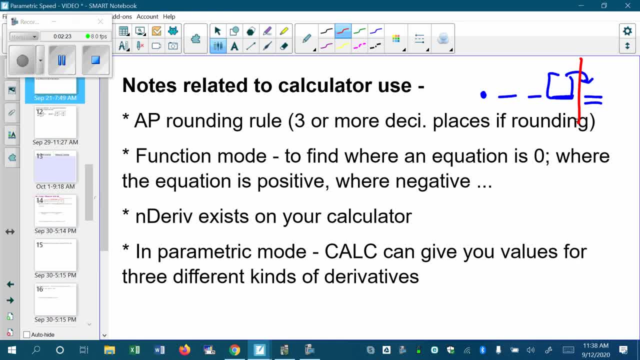 If you're just basically looking for an equation and like: what's the when is this equation equal to pie, that would be something you can do within function mode. right, You would graph the function. You'd graph: y equals pie. See where they cross, For example. 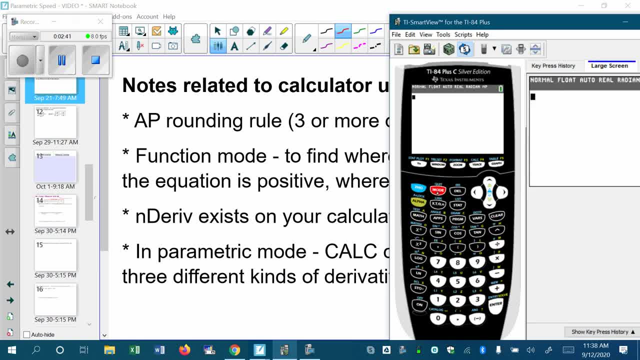 I had some students last year who did not know that this was a thing, or, you know, just get forgotten over the summer. So in the math menu I remember, 8 is the numerical derivative. Now again, there's your calculator. 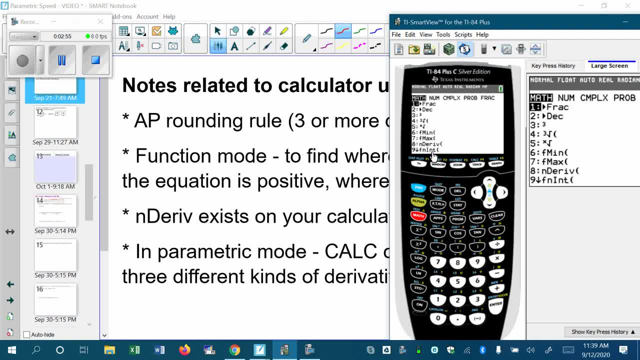 That's not actually no calculus, So what it does is to take 2 points that are very, very close together. I believe the default is 0.001 units, And so it'll take 2 points that are 0.001 units apart and find the slope of the secret line between those. 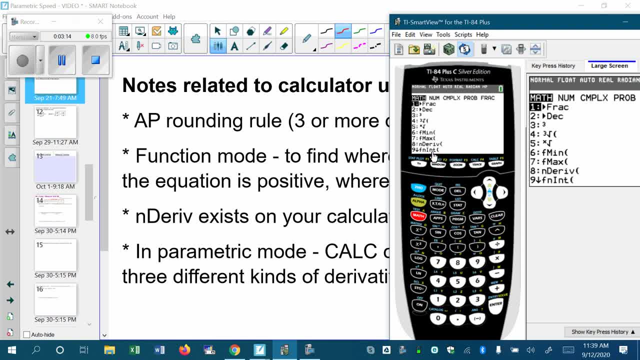 And that can be useful tool, just if you need to evaluate a derivative. So I just quickly put in here an example. So I'm in regular function mode. I have 5 x squared. I want to find, I want to find the slope of that function when x equals a particular number. So I can go into the math menu, I can pick item number 8.. I want the derivative with respect to x of my function. 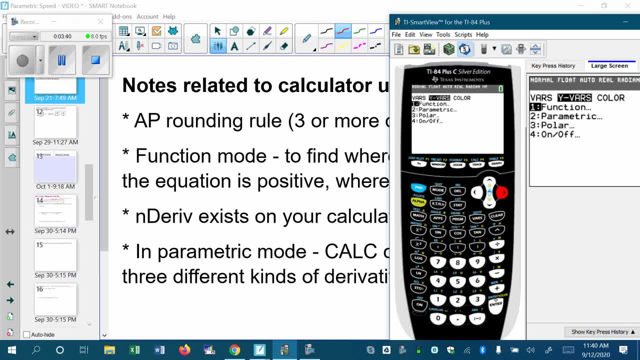 That is in the y menu y equals- it's my y 1.. I could certainly do that by typing in the equation itself, but if I already have the equation in my y equals, especially if it's a very cluttered equation, I don't want. 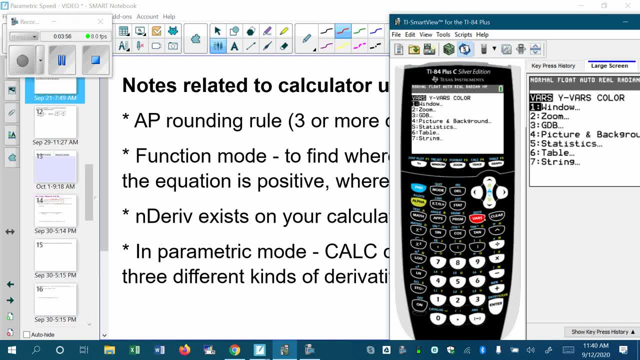 I don't want to type all that again. Are you kidding me? So there it is, Why variables function to that, Okay. And then come over here and say I want to know the soap when x equals 2. For instance: okay, it tells me that slope of 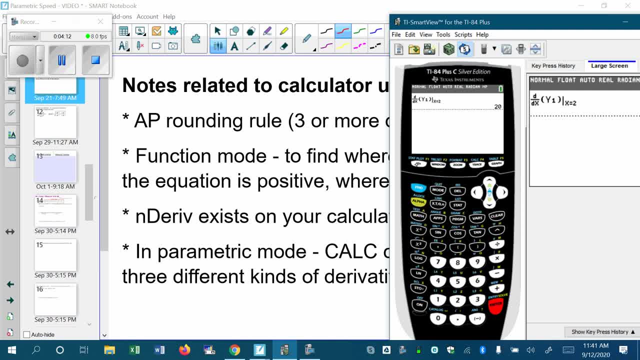 That graph at x equals 2,. I also can Come back into my graphic menu and utilize this in a different but similar way. So still fill in here, Still fill in y 1 here, but then say: I want this for all x values. and then, if I just do this on the standard window, it's going to give me a graph of the parabola and a graph of the derivative. 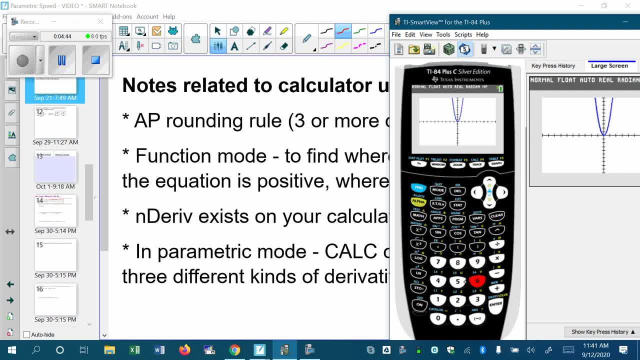 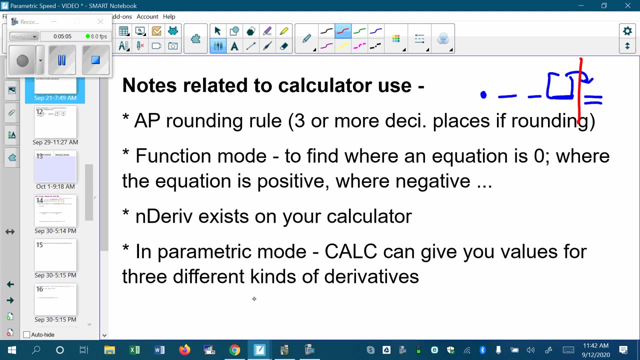 And that graph of the derivative will come up kind of slowly- Usually not this slowly. where where's my derivative? Oh, there it is. This is really slowly Back the derivative. now it doesn't give me the equation of that derivative, but it does. let me visually see the derivative. Okay, So I hope that you knew that from math analysis And if not, hopefully you know it now. 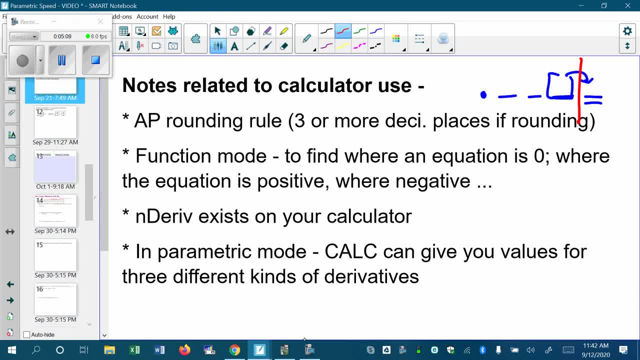 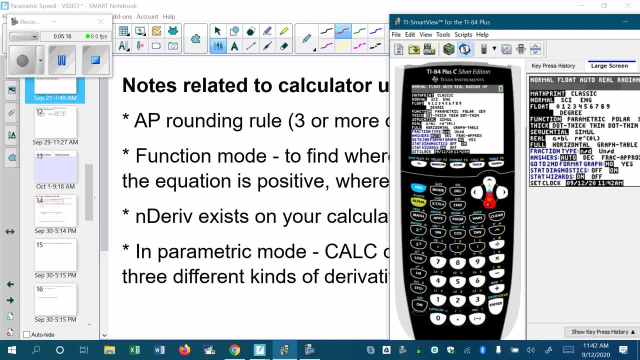 I also wanted to point out: in parametric mode, the top menu can give you some more things, So let's go back. I had this example from the other video that I recorded in this unit, So you might recognize the graph. Oh, now I changed my window. Okay, I just wanted to be able to see this a little bit better, especially if you're watching on a phone. 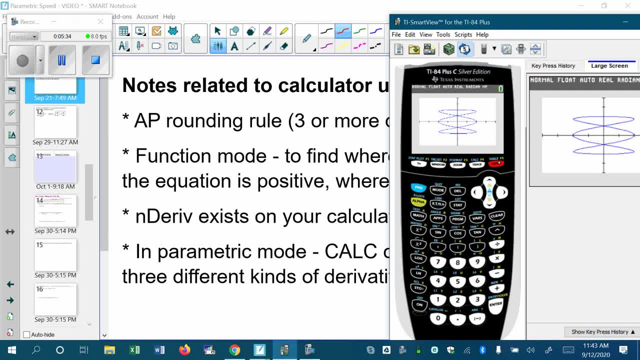 Okay, so that was that on parametric graph. that was in the previous video. If you look in the calculate menu- Look at this, isn't this nice. You can find a value, You can find a slow. all the 1st order derivatives are right in there. So if I had a question where I needed to find 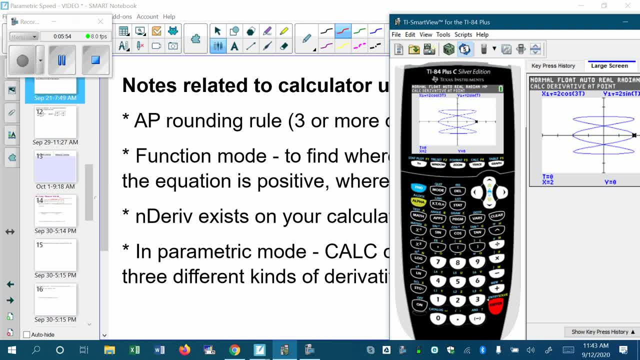 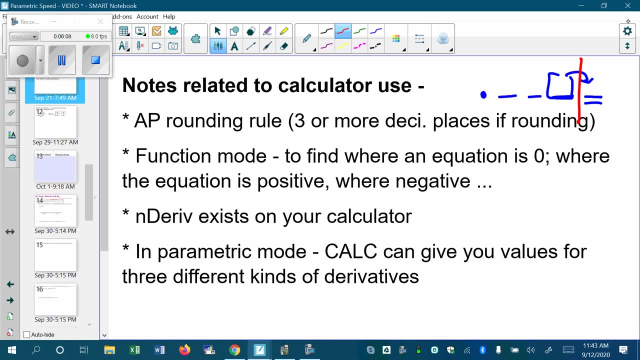 At a particular location- maybe I care about at pie over, for for my parameter It's going to tell me the slope and it's also going to visually locate that for me. Nice, right. So I hope you're in the habit of when you learn more math. 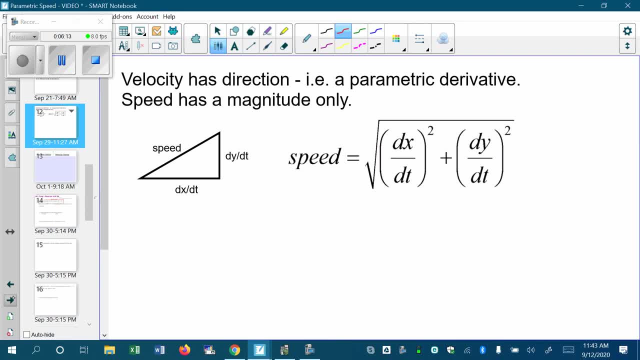 Thinking: I wonder if this is a calculator somewhere, because that's what you should do: You should look for things and then you should teach your teachers where things are, because maybe we haven't even found it yet. All right, so the actual lesson, the difference between speed and velocity is a small but significant difference. Velocity is what we would call a vector quantity, in that It has 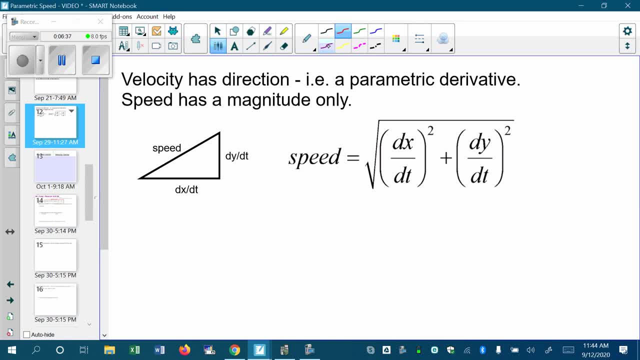 A direction to it as well as an amount. Okay, Speed is just that, Just the amount, so it's not taking into account direction. other than that, These 2 things are The same, but not really the same, because there's 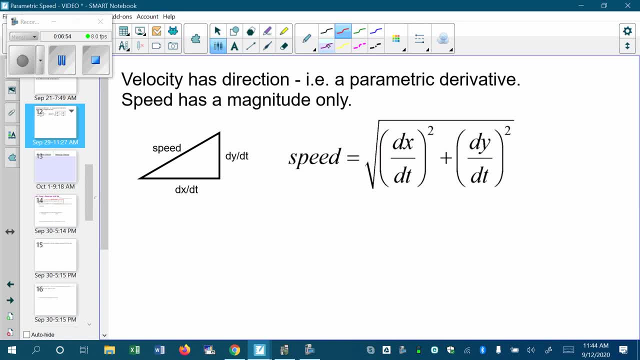 not the same, but same ish, right, We talk about the speed and then if we're talking about velocity, we say: well, it's the speed, but also taking into account if I'm going forward or backwards, or up or down or something like that. 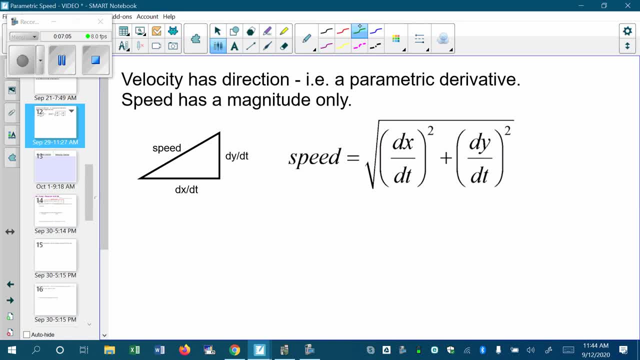 This little picture really is a very helpful little picture. Okay, Look at this guy. So if you think about this, it's just like a little rate of change triangle, rate of change, right Triangle- And think about: okay, horizontal rate of change. represent that on the horizontal vertical rate of. 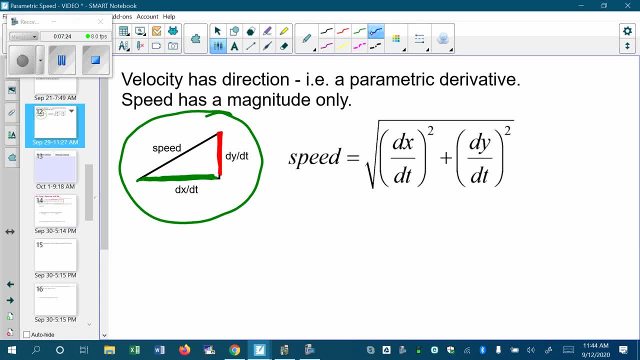 Change represent that on the vertical, then speed, since it is just an amount, not a direction, is the rate of change in that side of my little right triangle. And because you know, you could just say, well, I know that square plus square would be speed squared. 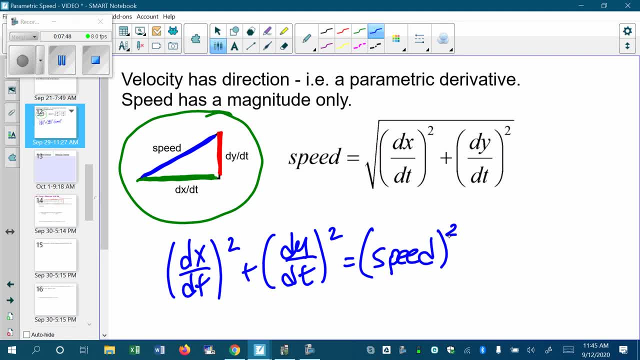 This is a little bit loose and free with the idea of link versus quantity, but Close enough. And then if I want to get rid of this square, I would square with both sides and then you come up with this. So I just think that this little picture- and I always can remember how I find speed in terms of parametrics- I'm going to look at that horizontal rate of change, I'm going to look at the vertical rate of change, And then it's basically just put diagram theorem right on top of that. 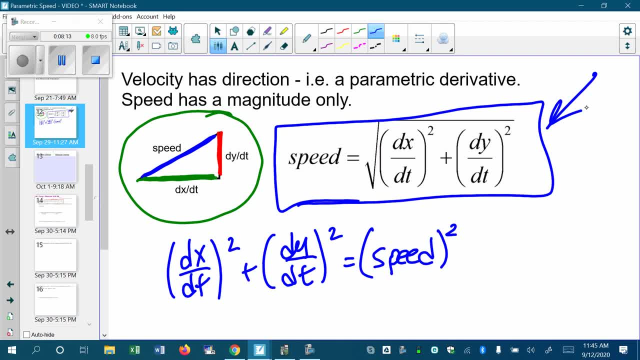 Now, something that I'd like to note at this point as well, just in my experience with teaching um BC- is: sometimes people are a little bit skittish about the word vector. Okay, that's just in BC, like really no big deal. because they do like there's a lot of vectors If you actually study them deeply, If you ever take a mathematics class, algebra- so much about vectors, Oh my goodness. 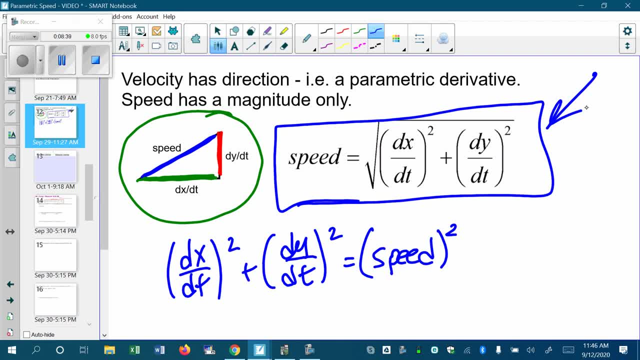 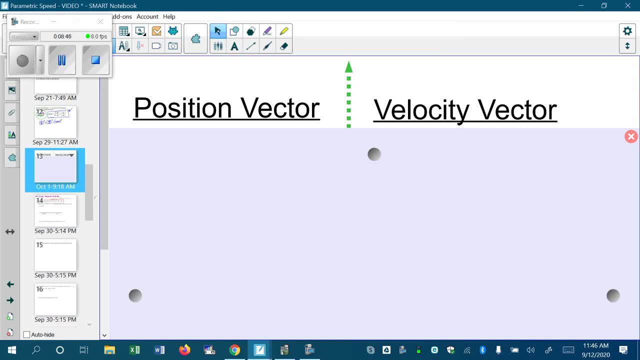 So there's a lot that could be there. The BC calculus Does not do all that, you guys, it's really, really chill. So when a question asks you about a position vector, velocity vector, The word vector, Okay, In BC life should just to you to put 2 components together with a comma and you can send some brackets if you want. but you don't even have to write a positions vector is: just where am I in terms of X? Where am I in terms of Y? 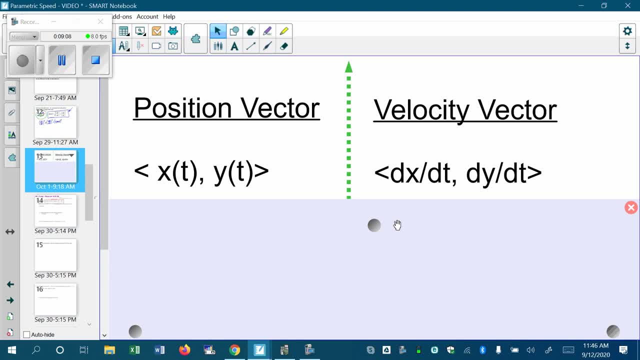 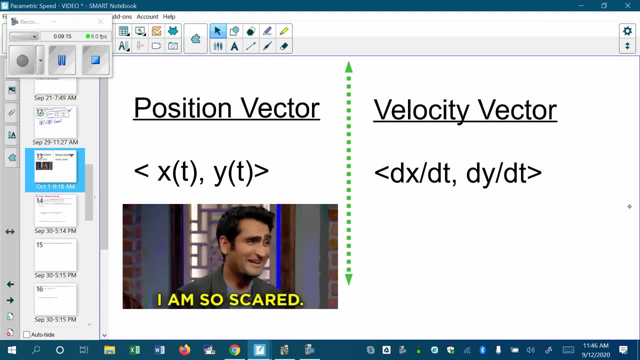 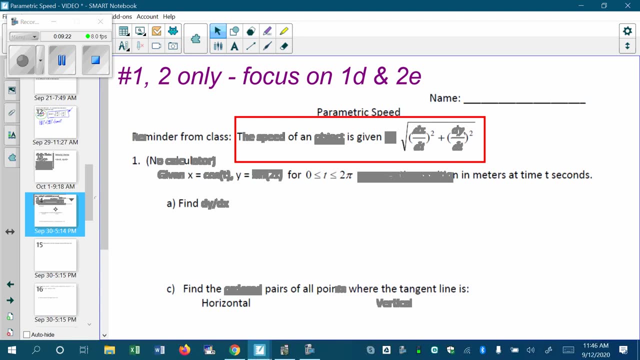 Put real brackets on velocity vector. rate of change in X, rate of change in line. Put the fancy brackets on it. That's it. You do not Need to be so scared. So today's lesson, it can be encapsulated by that red box that's on the screen right now, and I am going to, in particular, focus on just parts 1 D and 1 E. big time, We'll do a little bit more than that. 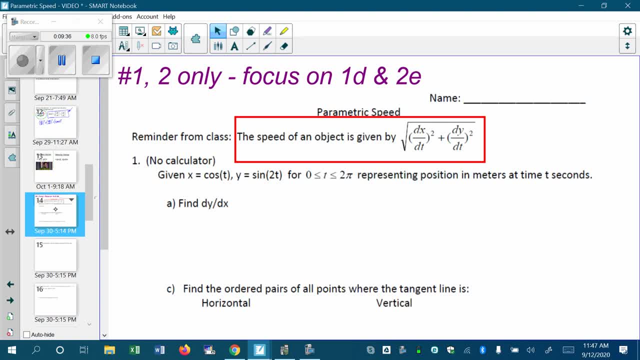 But 1, D and 1 E are the parts that are about speed, So I'm going to read this up to you. If you've been feeling really solid on parametrics, I give you my endorsement, my permission, my blessing to kind of skim through the video until I get to 1, D and 2 E, And you need to watch those parts, Okay. 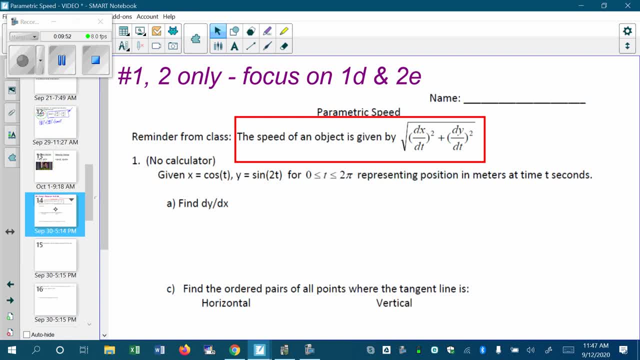 I'm just saying all right, but because that's the new, that I will go through all the rest. So if you're not doing so confident, you should say, on, watch the rest. Okay, Have a good time. right It's. I'm recording this on a rainy day. I hope you're watching it on a rainy day, Not a nice sunny day. But if you are watching it on a sunny day, Well, 1st of all, great, because it's a sunny day and that's enjoyable. 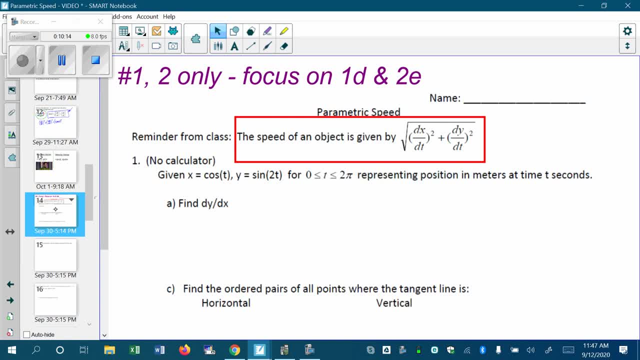 But you know, watch it as quickly as you can get it in your head So you can get some outside time. I'm just putting that out there. Okay, We're going to do some math. I promise I'll stop. 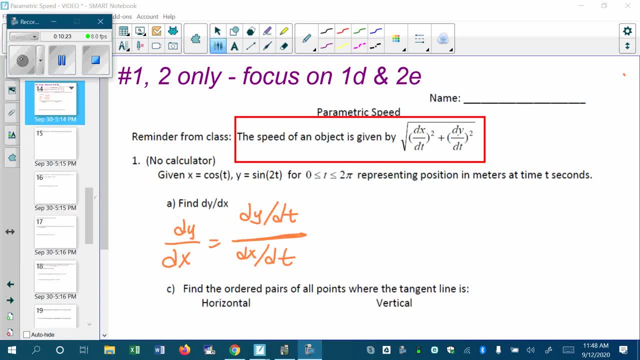 Boy, okay. So in 1, a, I'm going to remember the parametric definition of- is divided by. I'm going to look here for my 2, for my parametric equations that I need. I will take the derivative of why, with respect to time, and say: well, that's 2, cosine 2 T. this 2 is because of chain. 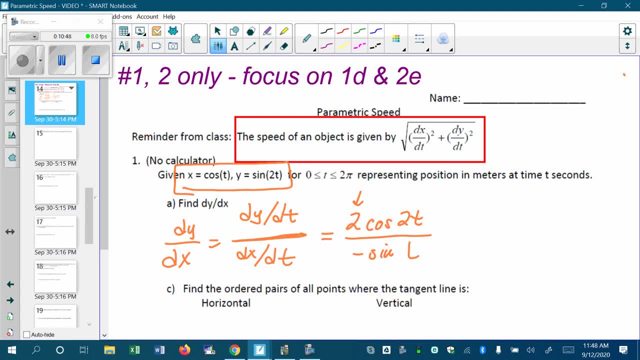 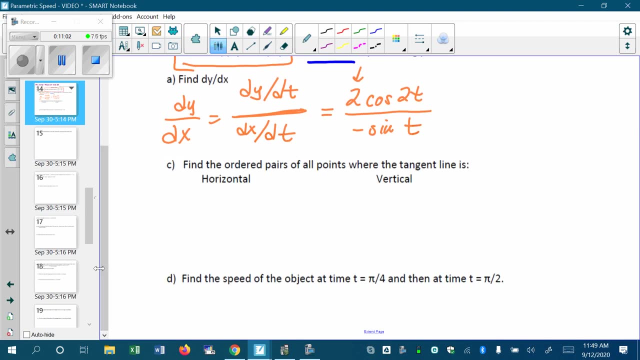 On the bottom, my derivative of cosine is negative sign. I noticed that I have a restricted Domain, so I only need to be thinking about this 1 time around the unit circle, so to speak. Okay, Then I'm going to come down here to the next part, where it asked me about the horizontal and vertical tangent lines. 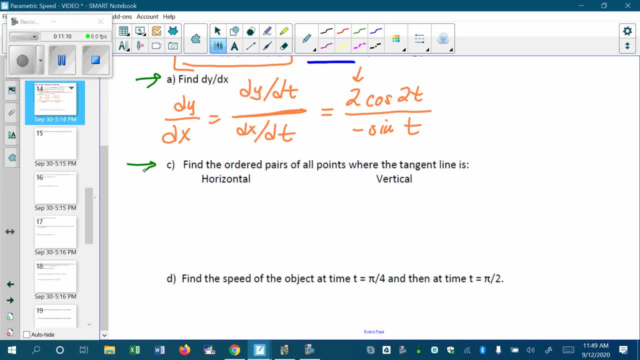 This entire sheet is totally like mislabeled with things. I'm just putting that out there every year, Like I've used this sheet before, every year I forget to fix it. You can be flexible, I think. I think Okay, So why is it that I wrote that Cosine of 2 T has to be 0. 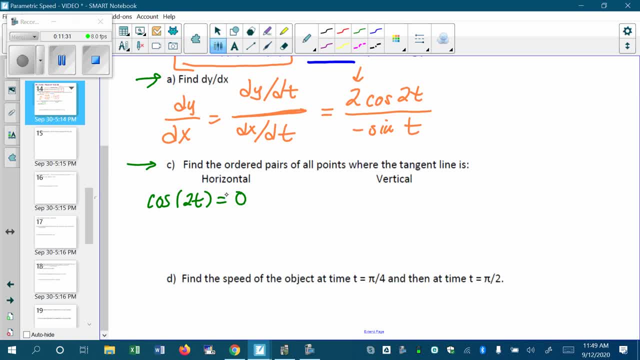 Well, if I have a horizontal tangent line, that means my slope, my, is 0, and if is 0, that means that this part has to be 0.. and so if that part is 0, that means that part is 0. 2 can't be 0.. the 2 in the front makes no difference. 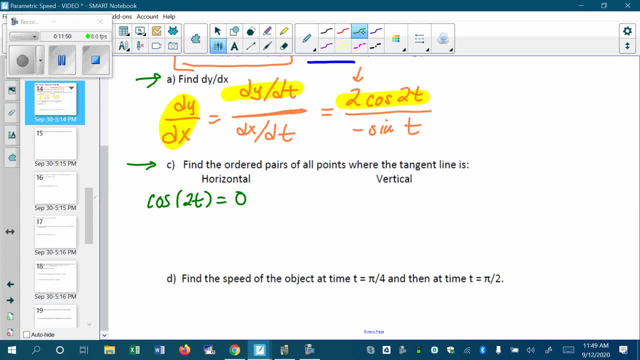 So it's really the other factor that has to be the 0. So I just need to know where cosine of 2 T is 0.. so I think about that, Think about my life, and 2 T is going to be at top of the unit circle plus. 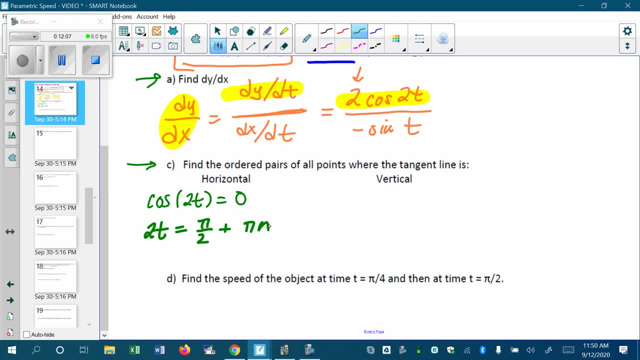 Bottom of the circle plus the top of the unit circle was the bottom of the unit circle Right. So that's pi units apart. So pi times N, and then, because of this 2 over here I'm going to divide through. 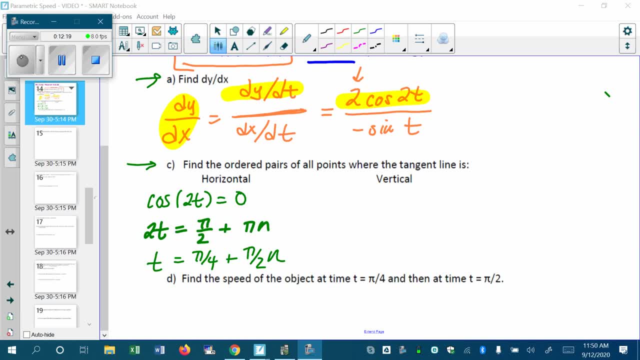 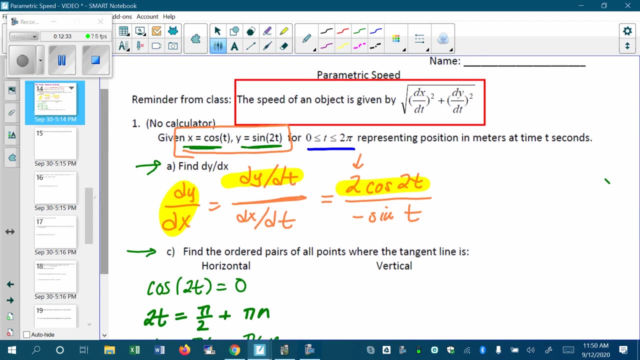 When I divide through by 2. I get pilot refer, And then increments of 90 degrees are at pi over 2.. so now, if I substitute in those values of T into my original equation, I can find the X and the Y coordinates that correspond to. 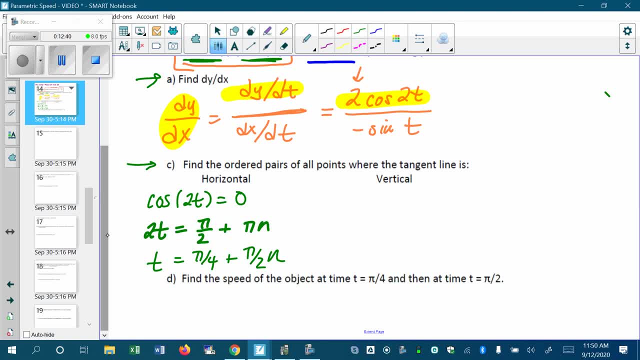 3 pi over 4 or 5 pi over 4, except from that, you know what I mean. Like, as you go around, so those ordered pay? Yeah, because that's what I know. Or here's are these. 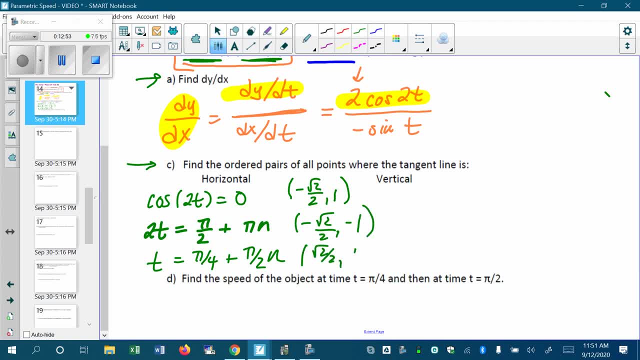 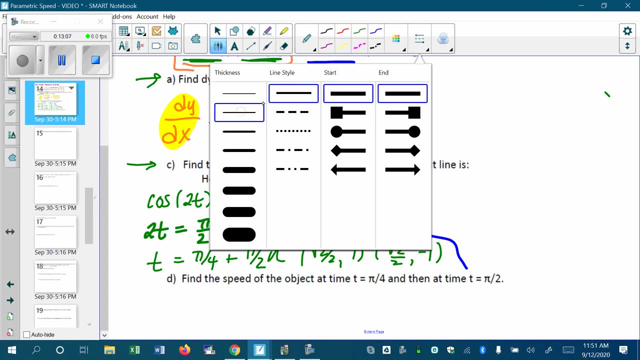 And then 2 over 2, 1, and then 2 over 2.. Okay, if you just substitute in that part, you just plug and Chuck. Okay, That's not like high For math, that's just evaluating. Okay. Then the vertical part is going to be: what happens when my slope. 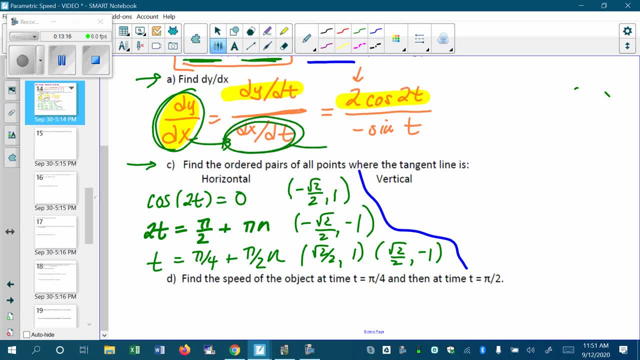 It was undefined, so this part is negative, which means that this has to be negative, which means that Sign of I just said negative, I meant 0.. Sorry, Let me try that again. So vertical is going to be when, this time defined, which means that this part is 0, which means that this part is 0. 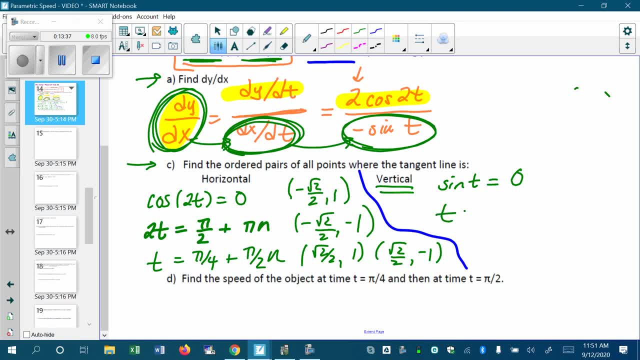 Okay, so sign is 0, sign is 0 at 0 pi, 2 pi, et cetera. Okay, So actually, you know I'm writing these in general and I just remembered I had a restriction up here that just went through 2. Pi. 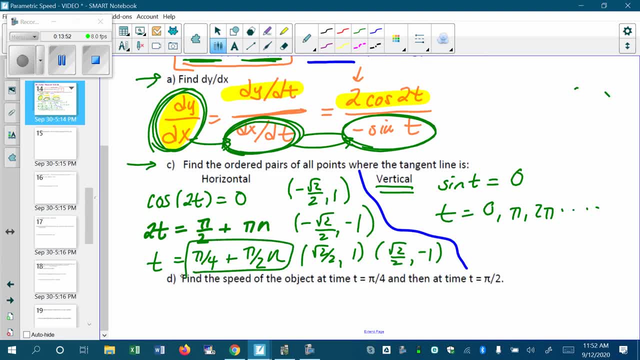 So you could have listed these out if you wanted to write instead. and this is going to stop. There's not going to be a dot dot dot, It's just going to be that. Okay. So Ordered pair. part from the previous question is still the same, though, So I'm going to plug in 0 pi, 2 pi. See what ordered pins I get. 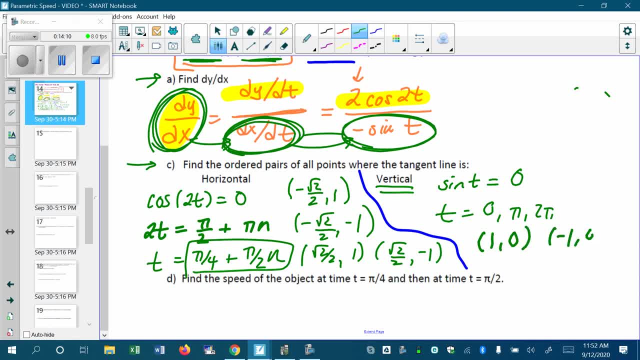 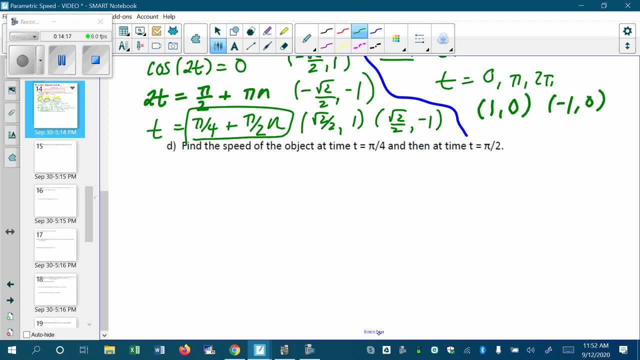 I get 1: 0 and negative 1: 0.. Okay Now, part D, I told you is 1 of the things that we want to focus on, because this is actually the new material, Right? So Here we are. important thing, Okay, From today. and I'm going to think about the fact that I have that little triangle and I'm going to remember that speed is that little triangle of speeds, of rates of change. 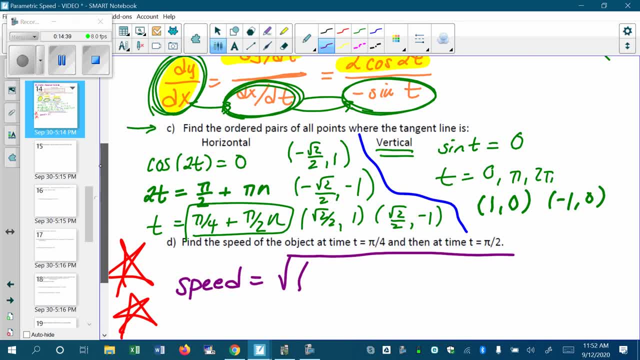 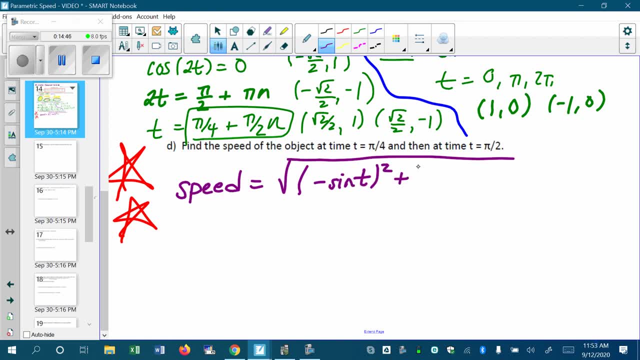 So I'm going to take my 2 derivatives- My was negative sign of team And my And I'm going to square those And take a square root. So that's my formula for speed. So if I want speed at a particular time, it's again a plug and chug. See, this is actually not that bad of a lesson. I'm just saying, like it's, it's really a formula. Okay. So I evaluate this at pi refer. I evaluate this at pi over chip. 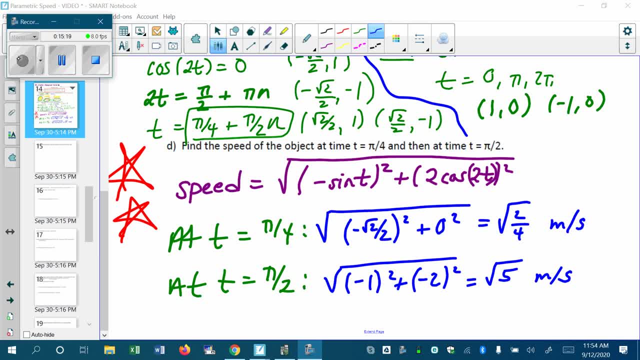 Okay, Okay, so that substituting in would give me the square root of a half or the square root of 2 over 2, something like that- meters per 2nd, depending how you wrote it. if you wanted to decimal there, like we talked about, you could have a decimal. make sure you have 3 decimal places that are accurate and same. on the 2nd part, you could have square to 5, or you could round that to a decimal: 3 decimal places of accuracy. 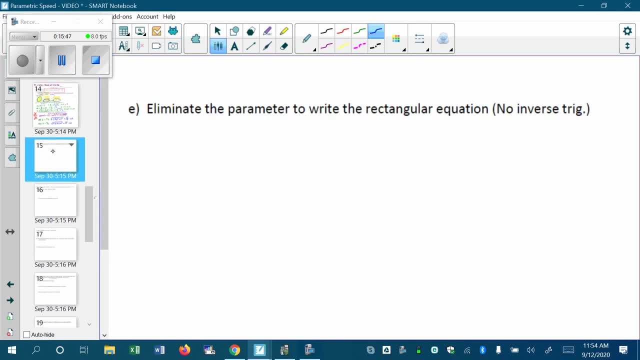 Okay, part E says to eliminate the Parameter to write a rectangular equation. Okay, So in this 1, I'm going to write down what my 2 equations were. So in the green and the 2 equations in the problem. 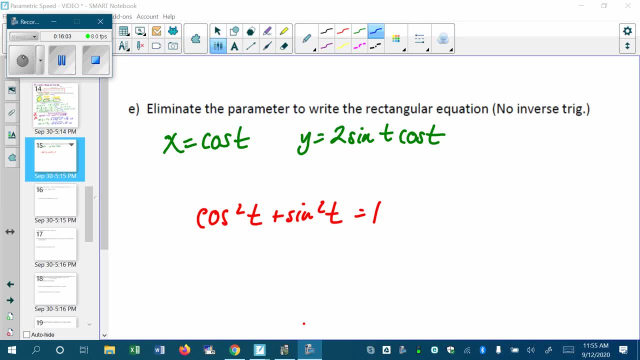 Or I never know if I should call this 2 equations or 1 set of parametric equations. I think it's more precise to say 1 set of parametric equations, because you need both of them to define the graph. Okay, So I'm writing down 1 set of parametric equations in green. 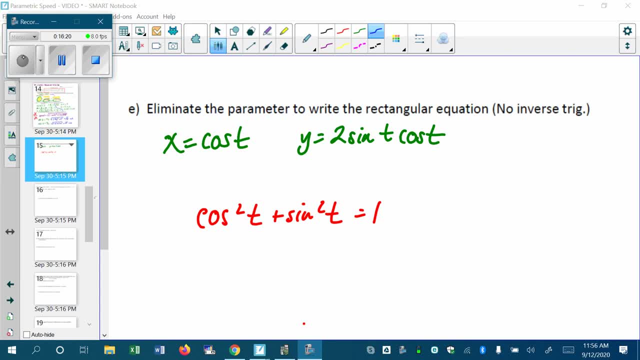 Okay, And then in red, I've written down the identity that I think I'm going to make use of, because I can see that both of these are mentioned, like sign and cosine, and red is a fact I can use to get myself out of parametric. 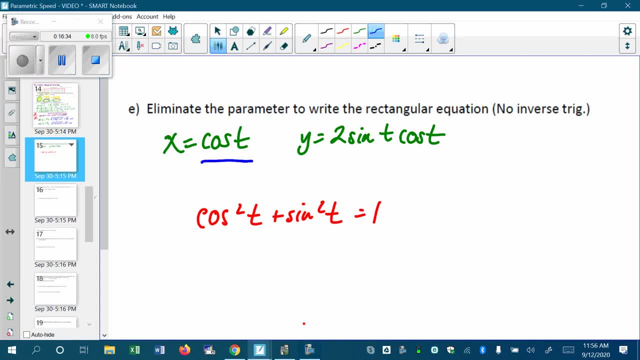 So this cosine of T is equivalent to X. So I'm going to put right in here that this is X squared. Now I need something else for sign, but over here I have something that mentioned sign. So I know that Y divided by 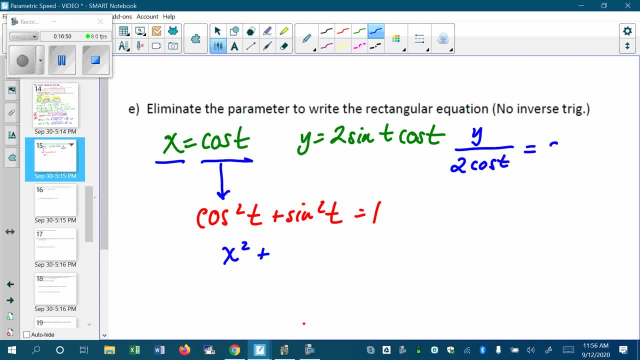 2, cosine of T is sign of T. and then I'm going to do a little loop thing here and say: well, X is the same as cosine, So I know that Y over 2 X is sign of T. And now I have something that gives me something parametric as related to something rectangular, And that was my goal. So in place of the sign of T in this identity, I can replace: 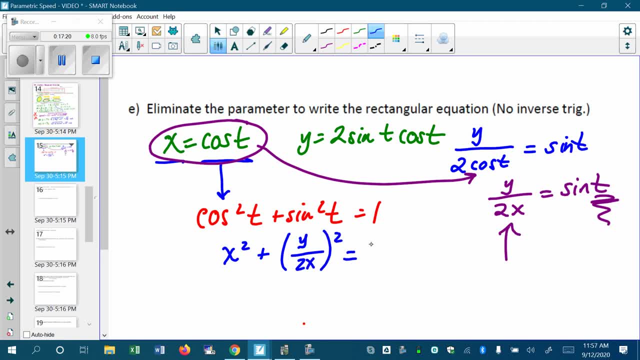 That with this rectangular form statement, and then I'm good to go. I could tidy that up if I want or not, Because calculus Yay. Okay, I actually think I might just skip now. Oh no, we should do 1 that has a 2nd derivative. Okay, We're going to do. 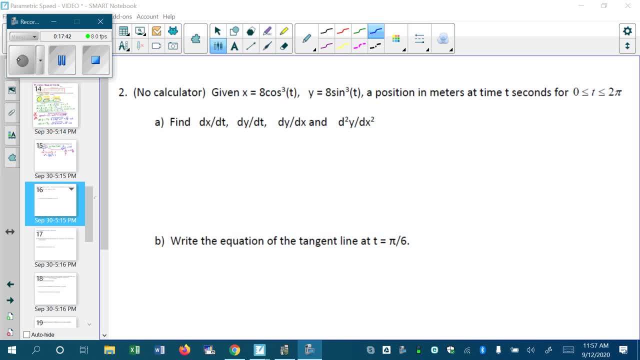 In fact, for 2,. what I'd like you to do is to write out those derivatives and come back and check your answer and, for to be, I'd like you to do the same. I'd like you to do the same. I'd like you to write the equation of the tangent line. tangent line, What do we think? 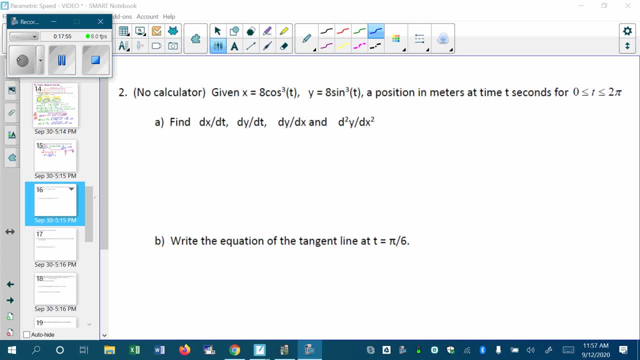 I need a point and I need a slow. Okay, So I want you to do and B, and then we're going to come back and do together and that's going to be it. This is getting a little on the long side, Okay, So we'll do 2 and B and then come back and do together. 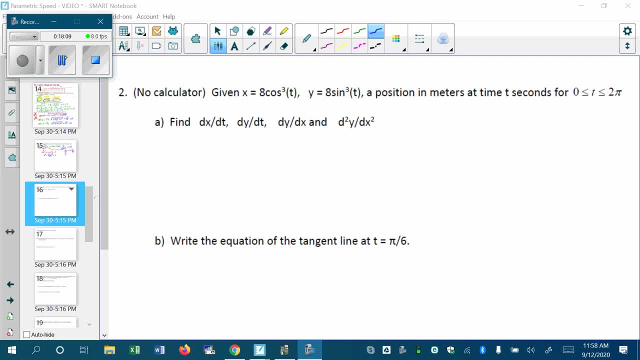 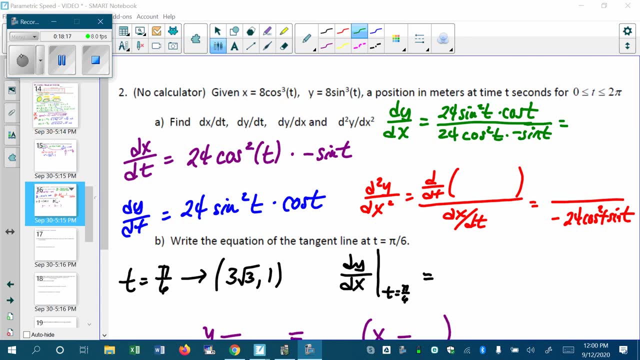 Try it and be by yourself now. Okay, I hope you tried this yourself. That's how you get practice. So 2, a: you find The rate of change in X with respect to the rate of change in Y with respect to T. make sure you remember that this notation from trig world really means in, respectively: cosine of T- quantity cubed, and sign of T- quantity cubed. 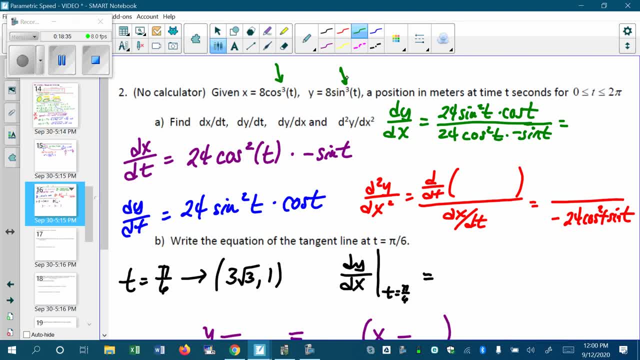 Okay, so they would have to treat it like that Right Use chain. We'll bring the 3 down in front, Keep the inside, take the insight to the 2nd and then multiply by the derivative of the inside. So that's where I got the purple and the blue. the green I have. 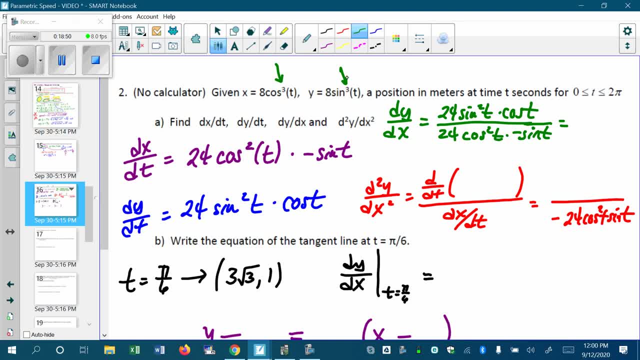 I've partially done. I'm taking the voting in blue and dividing it by the writing in purple. Okay, So when I set that up over here- that's where I'm looking right now- I get very excited because I get to cancel some things because they make 1.. 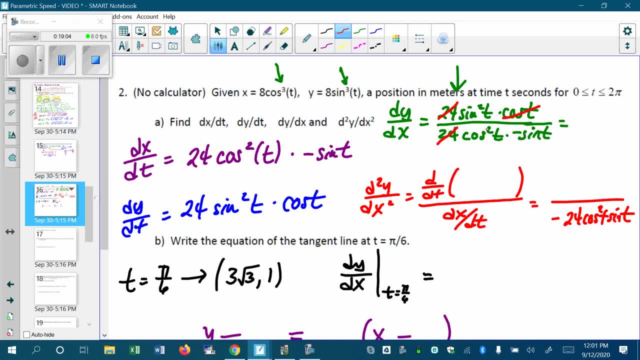 So 24 divided by 24 is 1 cosine. divided by another cosine would be 1 sign. divided by another sign would be 1.. I notice I have a negative here, So I'm going to make sure I don't drop that. And then all I have left is sign of a cosine. 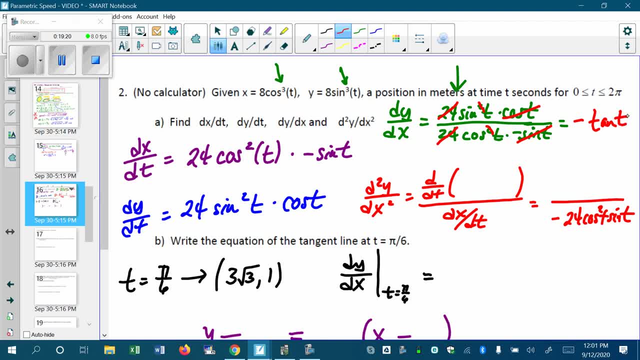 Which is tangent. so my slope is determined by the opposite of tangent of T. So then, remember from Mr covers video that the 2nd derivative is found by taking the derivative with respect to T of my D, Y, D, X, statement, and don't forget the critical piece of dividing by: 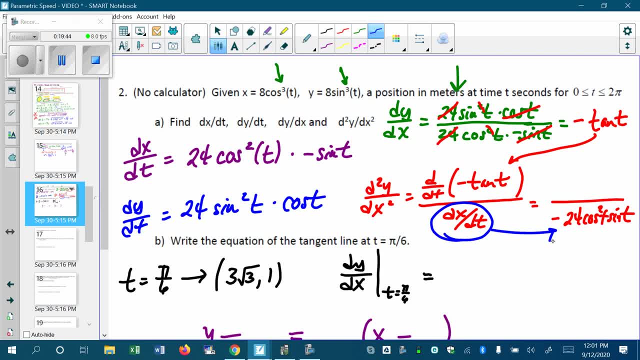 So here's my statement. I need to remember what the derivative of tangent is. The derivative of tangent is squared and my negative is just going to ride along. Okay, Now I could rewrite this: secant on the top is the same as cosine on the bottom, and the negative over the negative is going to make this all positive. 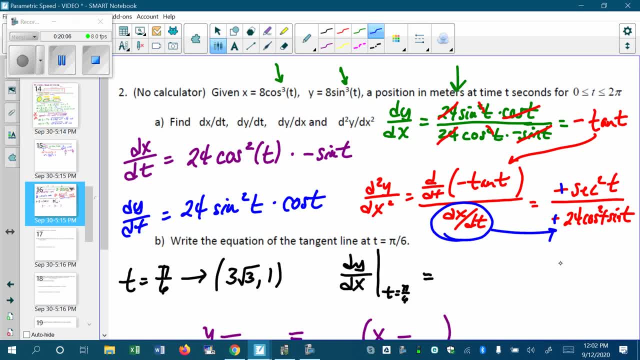 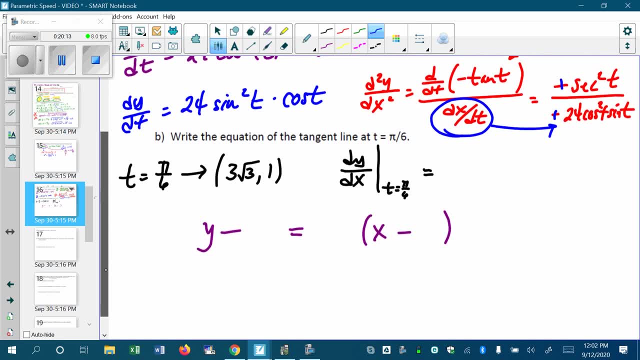 So you might have it as 1 over 24, cosine to the 4th time sign in the denominator. Okay, You might not, doesn't really matter. Okay, In this problem, if I need to, you write the equation at the tangent line. 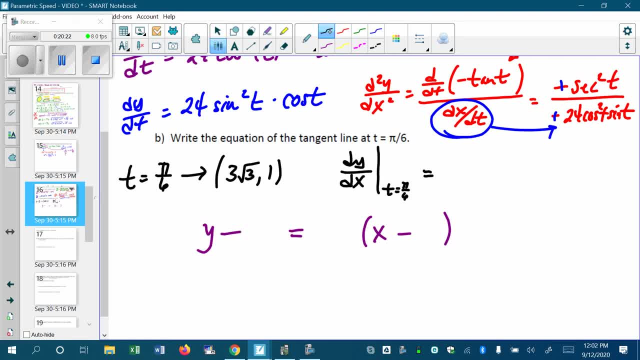 I need a point and a slope. So to get the point, I would plug in pie over 6 to X equals blank and Y equals blank, to find where X and Y each are. then I'm going to find my slope. So for soap. 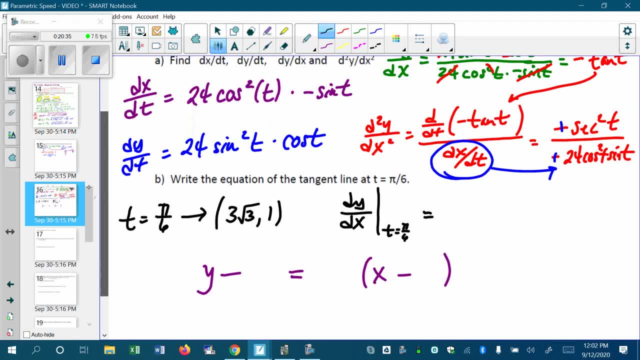 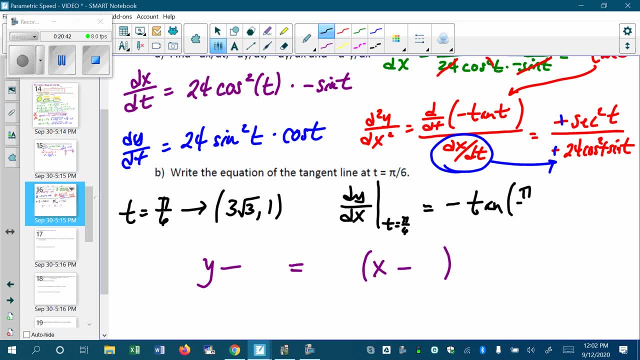 I need to use my equation from up above, which was opposite of tangent, And so I need the opposite of tangent at pie over 6.. My stylus is acting up, so note some things here. Uh, about notation. This part means at a certain value. that is the proper way to write it. 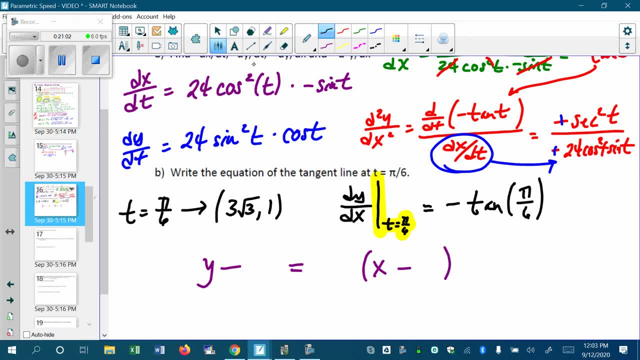 You can also use English right, Use letters at blah blah, blah, Right. But I shouldn't just be saying equal sign negative tangent of pi over 6, because that would imply that the slope is always negative. root 3 over 3.. 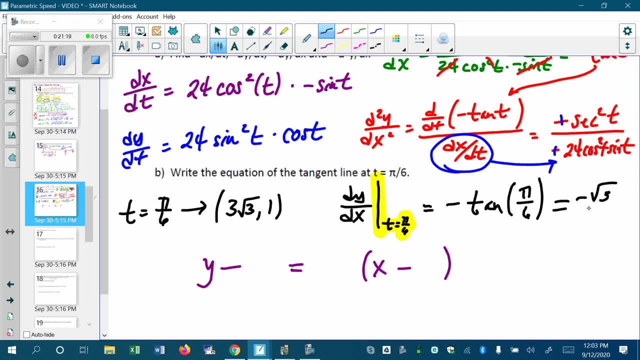 Whereas it is Not the case. this is just at a particular location, that that's the slope, and so I'm going to write here my slope, I'm going to fill in here my point and that was my point. slope form of a line. Okay, 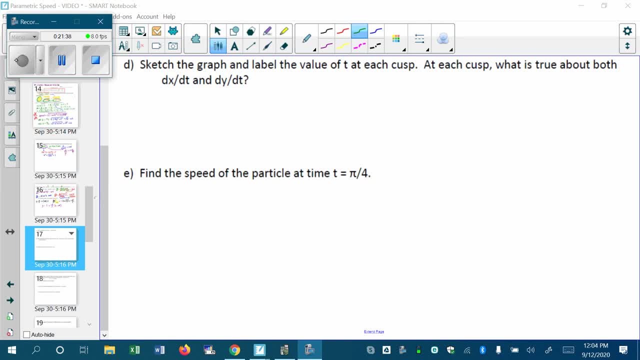 the last question I would like you to try is number 1, part E. So this says: find the speed of the particle at time equals pi over 4.. We're still within the same question, So we're still using the same pair of parametric equations. 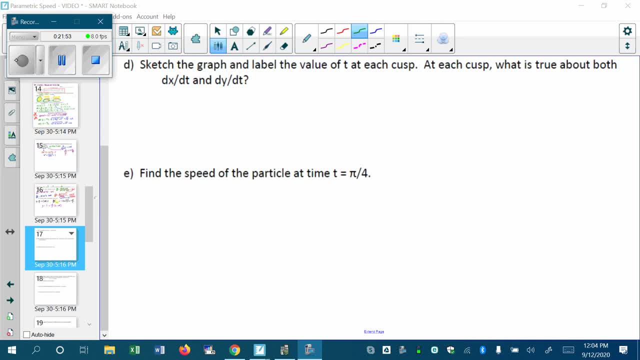 Okay, the same 2 that we were just working with. Okay, pause the video again and come back in a 2nd. Okay, hopefully this worked out just awesome for you. You get a really pretty answer. You just need to substitute in for your and your, make sure you square both pieces and you should end up with the square root of 1..